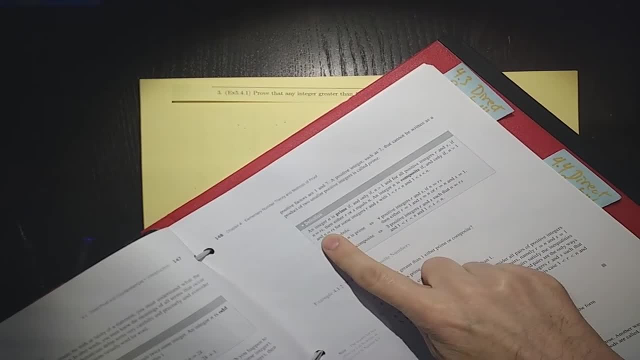 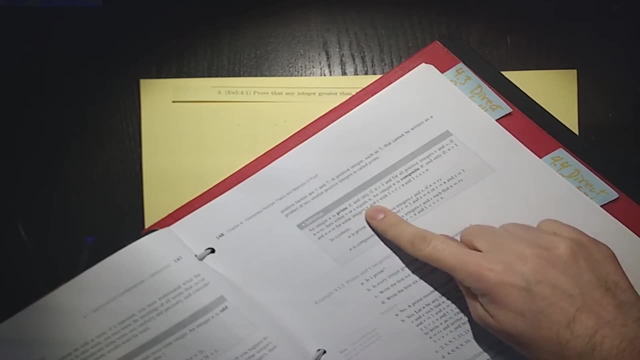 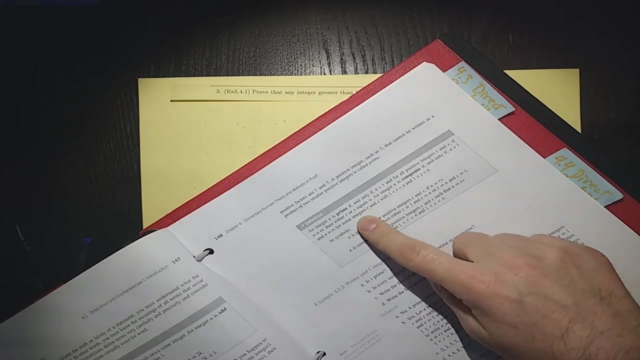 And for all positive integers r and s. if n is the product of r times s, then either r or s equals n. And what happens if that's not true is that we call n composite, that n equals r times s. for some integers r and s. 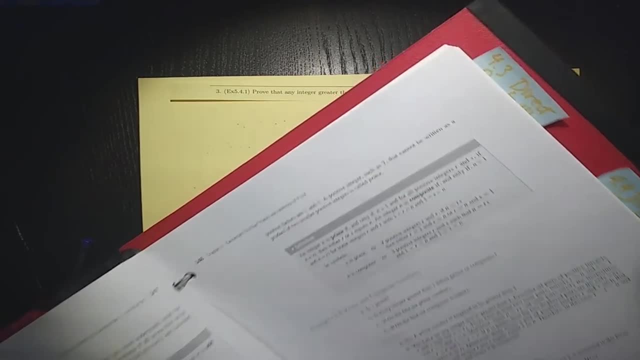 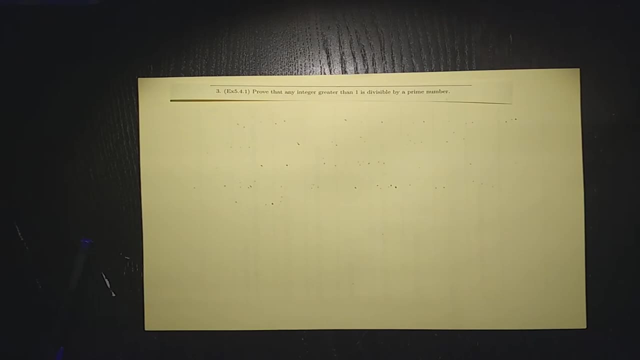 and neither r nor s is equal to n. They'd be in between. So that's the definition of prime, and we need to show that every integer greater than 1 is divisible by a prime number. So what we can do is this: 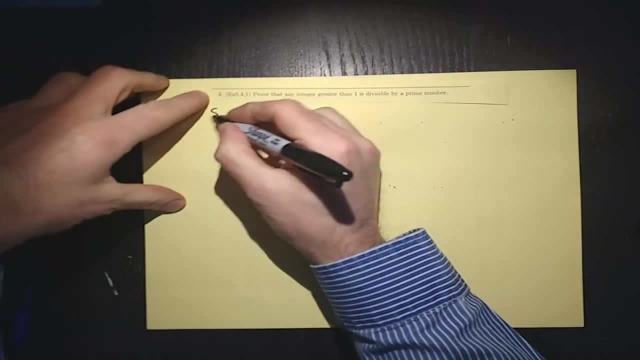 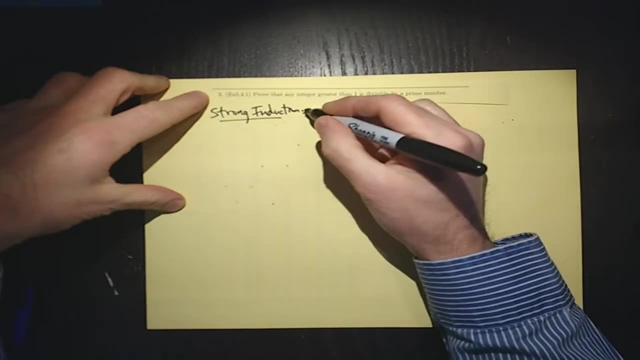 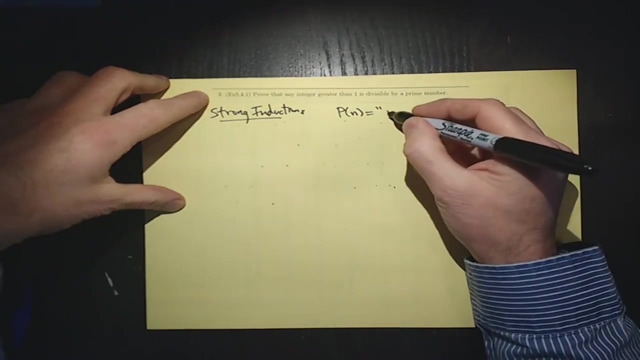 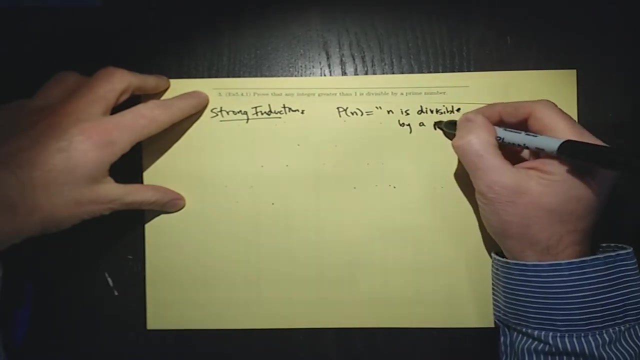 We can do a proof by strong. We can do a proof by strong induction And, of course, we need a statement. We need our p of n. p of n is the statement that n is divisible by a prime. And so when we do this, 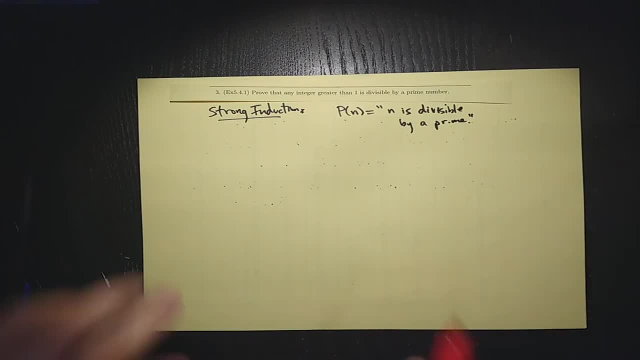 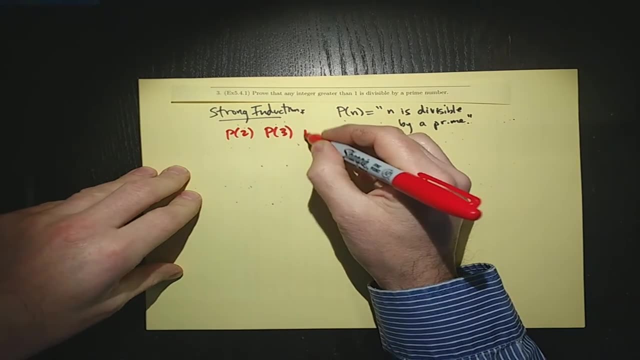 we want to prove that p of. we actually want to prove that p of 2 is true. We want to prove that p of 3 is true, That we want to prove that p of 4 is true all the way up to p of k. 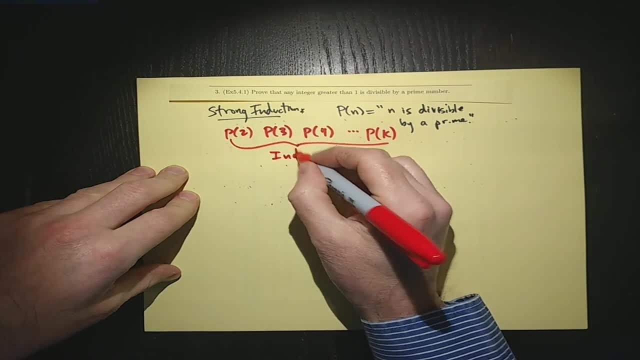 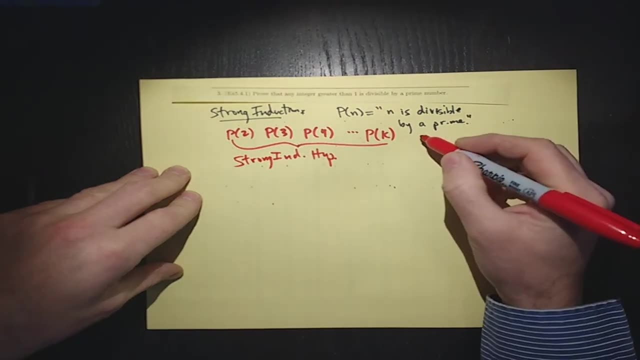 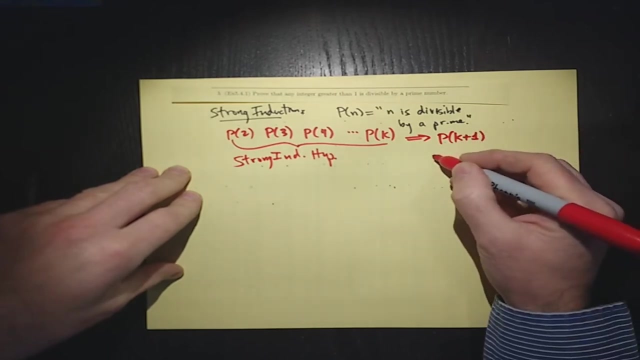 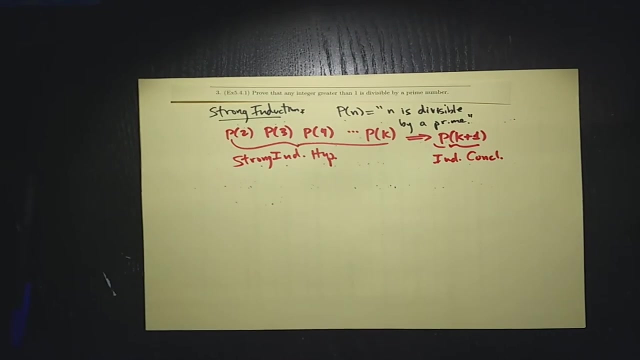 That's our induction hypothesis, Actually that's our strong induction hypothesis, And then that should prove that p of k plus 1 is true. This is the induction conclusion, although nobody calls it that except for me, But we're going to suppose. well, once we've done the base case. 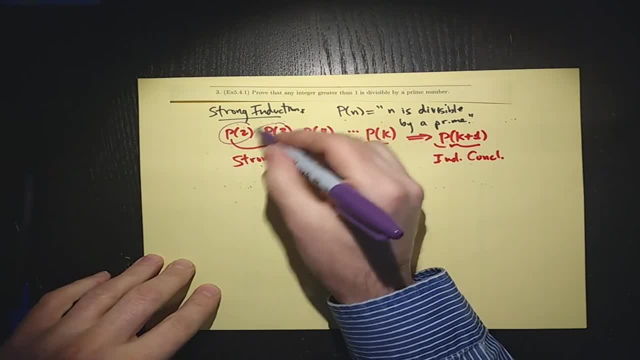 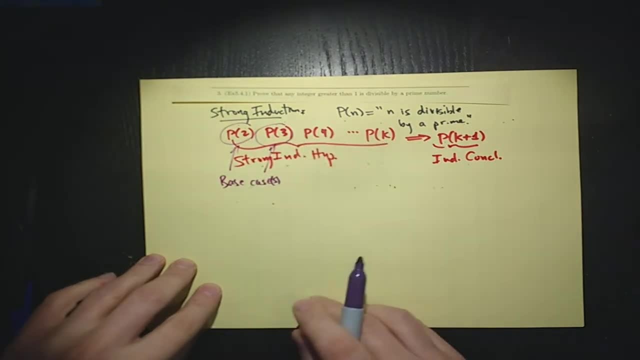 the base case. we could use this as a base case, or maybe these two base cases have a p of 2 and p of 3.. Notice that it should be n greater than 1, so we don't want p of 1,, we want to start with p of 2.. 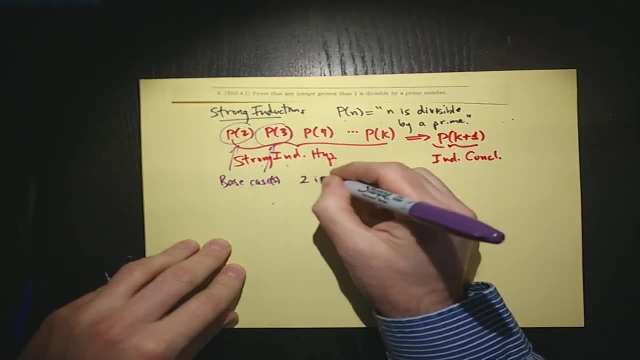 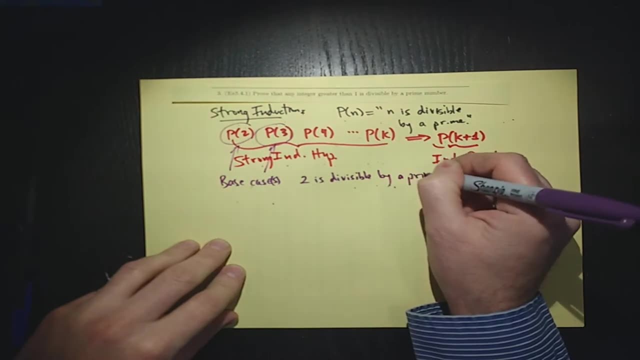 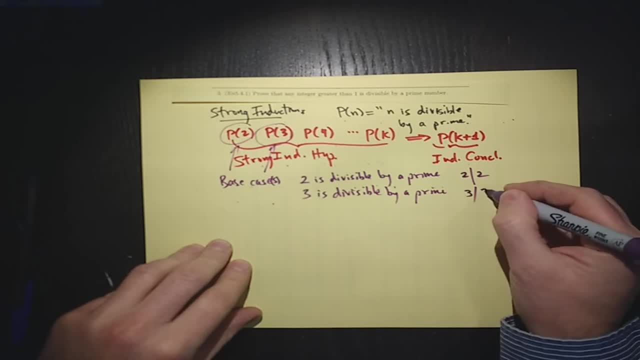 Well, 2 is a prime, so 2 is divisible by 2.. And 3 is a prime, so 3 is divisible by 3.. We could even continue. You don't need to limit yourself to one base case, but most people do. 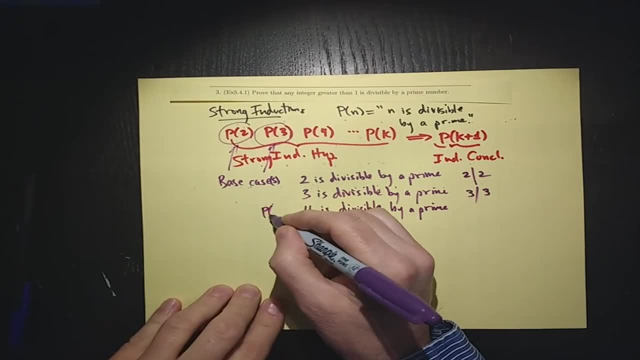 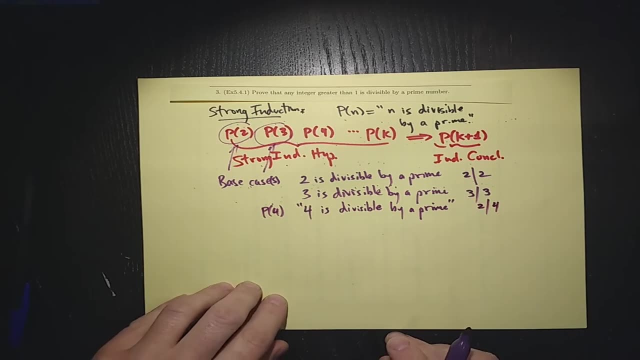 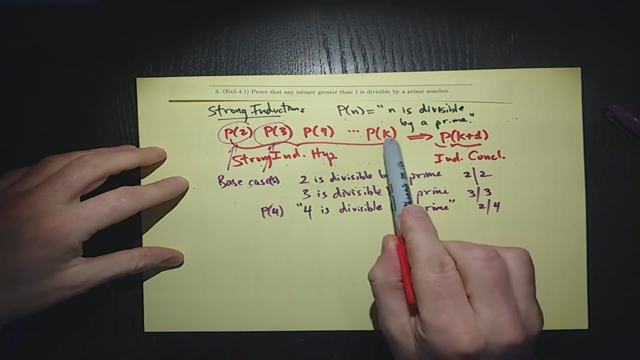 But p of 4 would say that 4 is divisible by a prime, and of course it is because 4 is divisible by 2.. So let's suppose that that every number between 1 and k is divisible by a prime, and we have to show that k plus 1 is divisible by a prime. 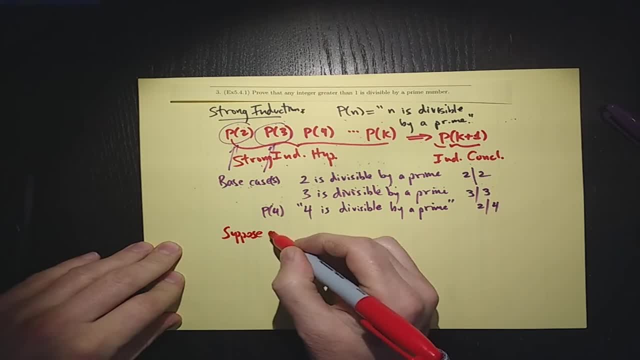 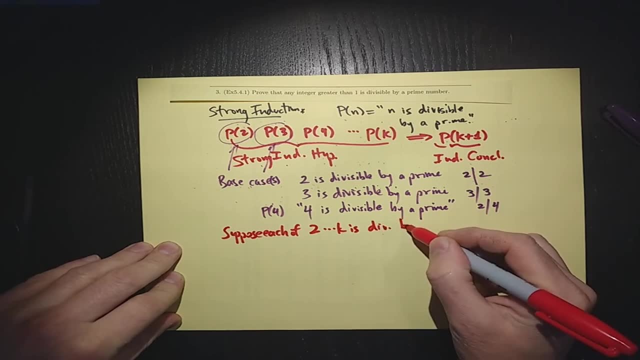 So suppose each of 2 up to k is divisible by a prime And we're going to consider k plus 1.. Now there's actually really two cases. Now there's actually really two cases. Now there's actually really two cases. One is the trivial case. 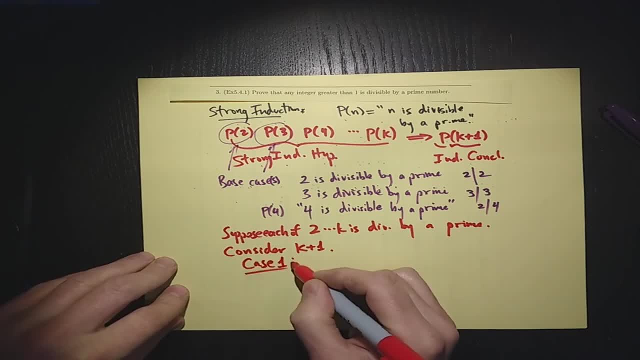 One is the trivial case, Case 1,. if k plus 1 is prime, well then just like 2 and 3, k plus 1 is divisible by itself. k plus 1 is divisible by k plus 1.. So k plus 1 is divisible by a prime. 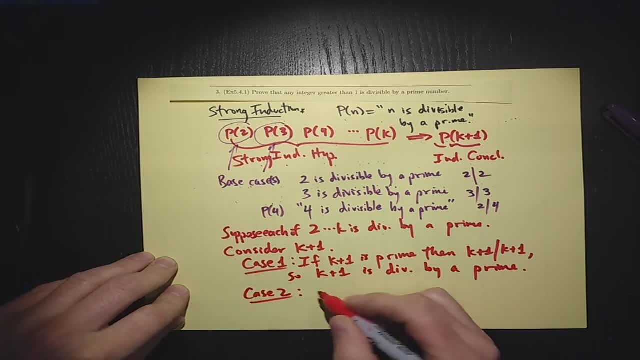 And we're set And now we need to do case 2.. If k plus 1 is not prime, then it's composite, And the definition of composite means that this k plus 1 is r times s, this k plus 1 is r times s.